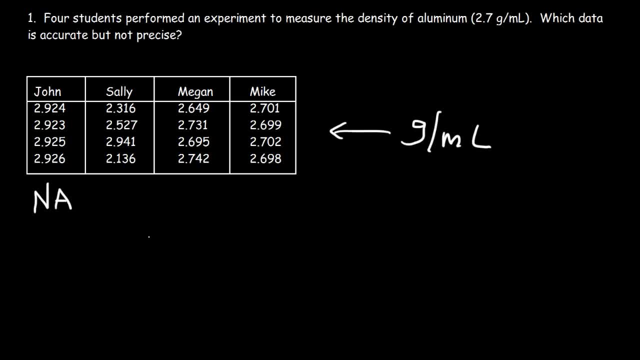 NA for not accurate. Now what about Sally's data? Is it accurate? Is it close to 2.7?? As you can see the numbers, they vary widely. They're not close to 2.7 at all. So her data is not accurate. Now what about Megan? Is her data accurate? 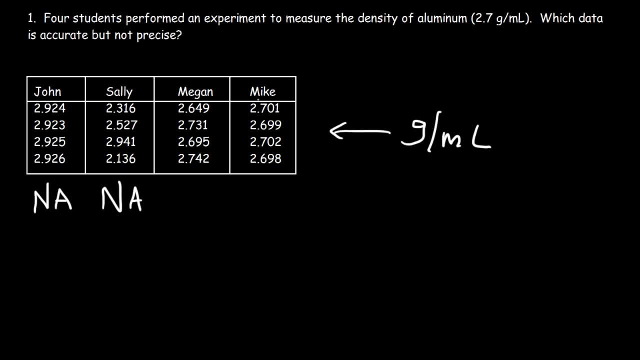 Now, relative to John and Sally, Megan's data is pretty close to 2.7.. 2.649,, 2.73,, 2.695, that's very close to 2.7.. So we can say that her data is fairly accurate, at least compared to John's and Sally's data. 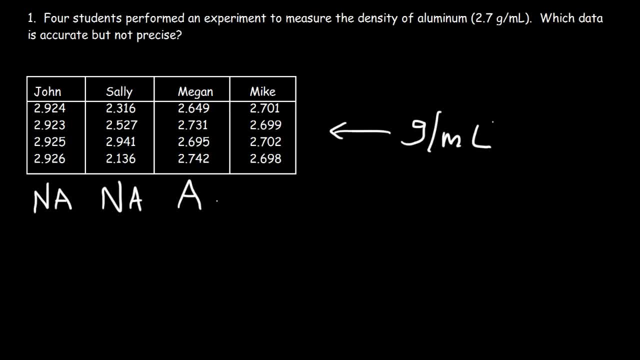 Now what about Mike? Mike's data is definitely accurate. It's very close to 2.7.. Now let's see whose data is precise. So let's talk about John's data. Is it precise? Do the values agree with each other? And it turns out they do. All of his values, each of his trials is around. 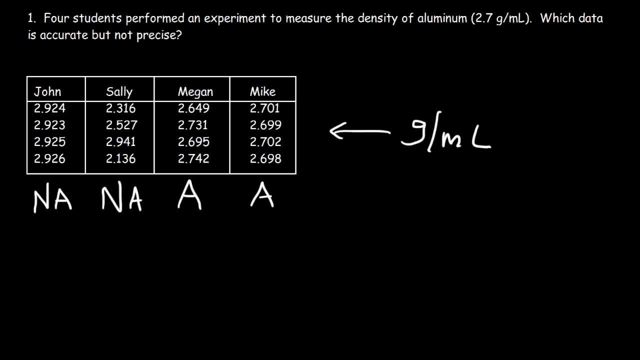 2.9.. 2.924, 2.923.. So those numbers they're very close to each other. They agree with each other. So John's data it's precise. Now, what about Sally? Sally's data is not precise. First it's 2.3, then it's 2.5, then it's 2.9.. Those numbers do not agree. 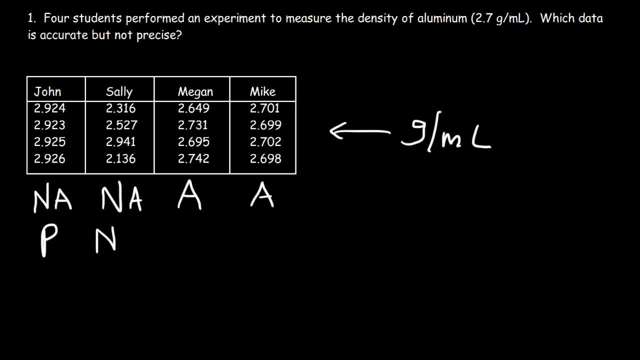 with each other. They're not close to each other, so it's not precise. And, Megan, it's her data precise. Her data jumps around too kind of like Sally's- Maybe not as extreme as Sally's data, but it doesn't agree with each other. First it's 2.65, then it's 2.73, then 2.695.. So it's not. 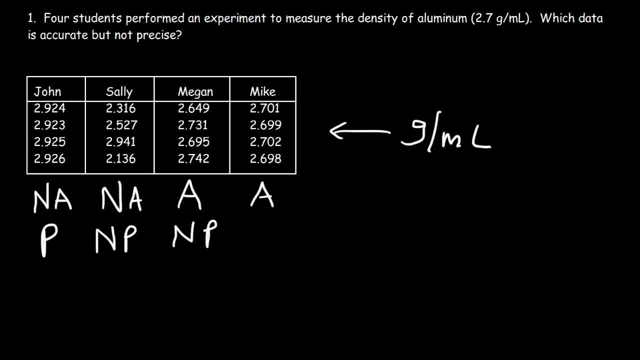 very precise. Now, Mike's data is precise: 2.701 and 2.699, that's very, very close. I mean the difference between the trials are about maybe 0.002 or 0.003.. So that's very close.